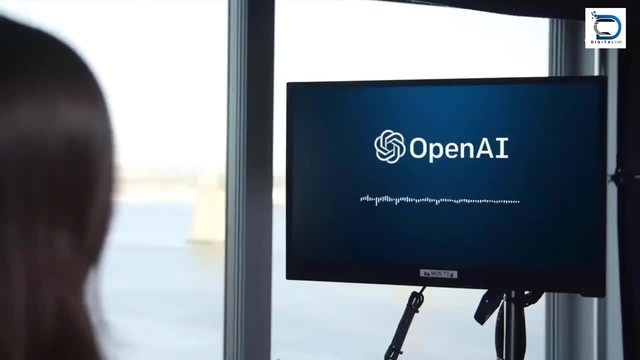 I am ChatGPT, a large language model trained by OpenAI. I am capable of understanding and generating text and can answer a wide range of questions as well as generate creative writing and text summaries. So that's a short intro of what is ChatGPT in its own word. 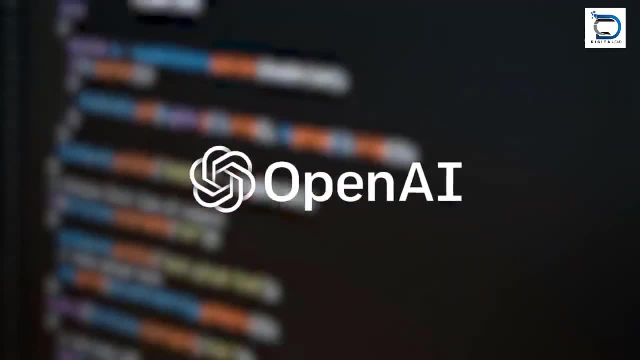 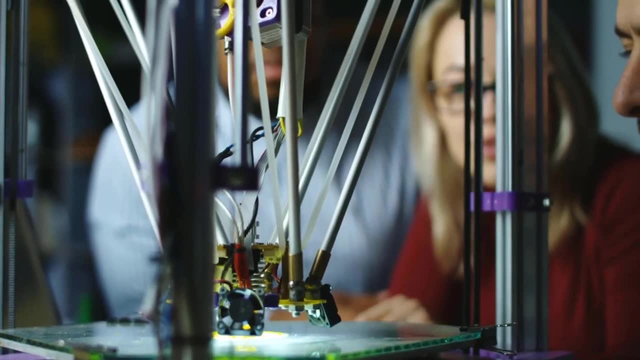 Let's see. ChatGPT is a language model based on GPT 3.4 architecture It is trained on. vast amount of data can assist in mechanical engineering in various ways. Let's start with research. Mechanical engineers often need to find specific information quickly and efficiently. 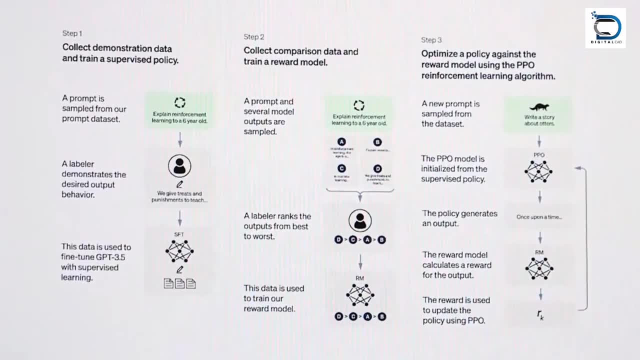 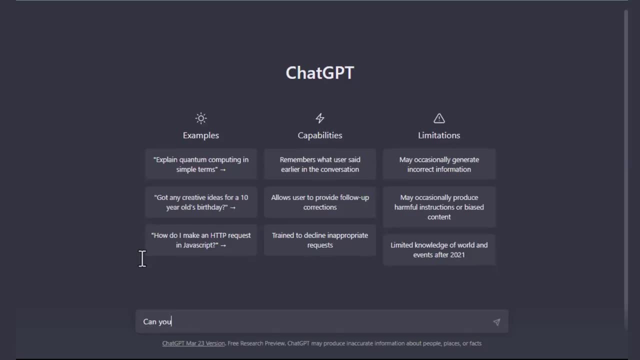 With ChatGPT, you can ask questions about mechanical design, material selection, manufacturing process and more. ChatGPT can provide a list of researches. You can also find a list of research results that match your query, allowing you to quickly find the information you need. just like the example, as you can see, 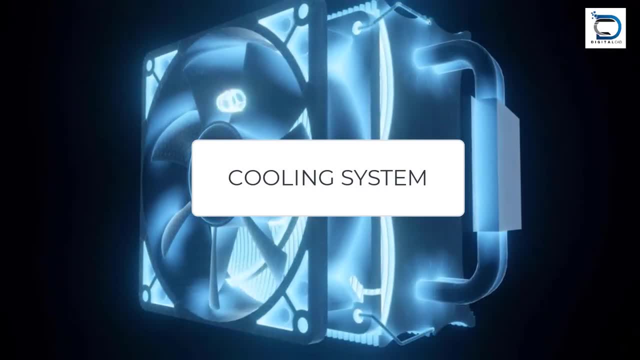 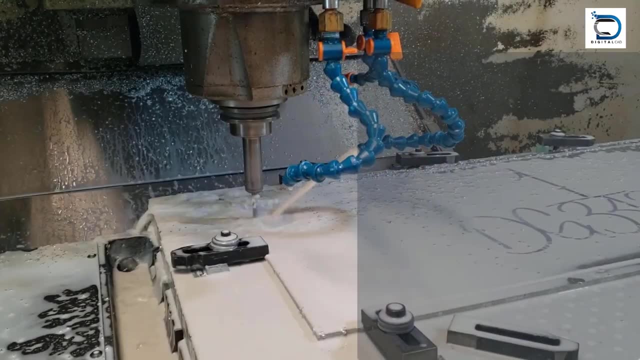 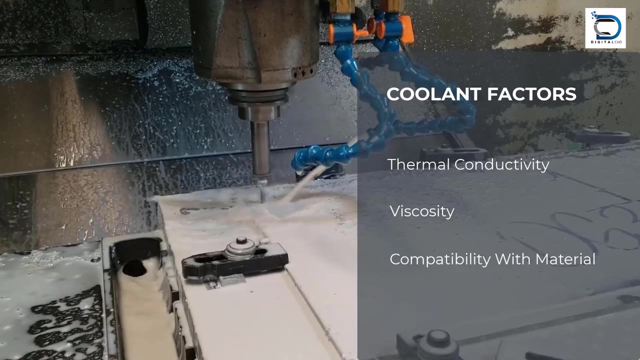 Let's take an example. Let's say a mechanical engineer is designing a cooling system for industrial purpose that involves a large amount of heat dissipation. The engineer needs to select the appropriate coolant for the system, taking into account factors such as thermal conductivity, viscosity and compatibility with the material used in the system. 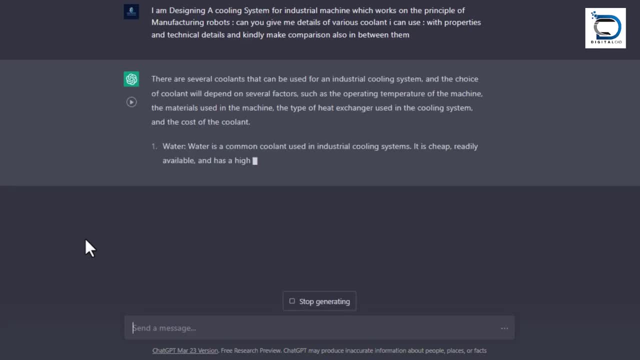 The engineer can ask ChatGPT to provide a list of research results that match your query, allowing you to quickly find the information you need. just like the example, as you can see, ChatGPT can provide information about the property of different coolants such as water, oil and refrigerant. 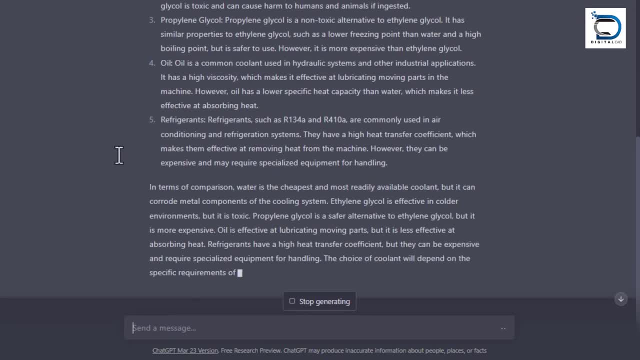 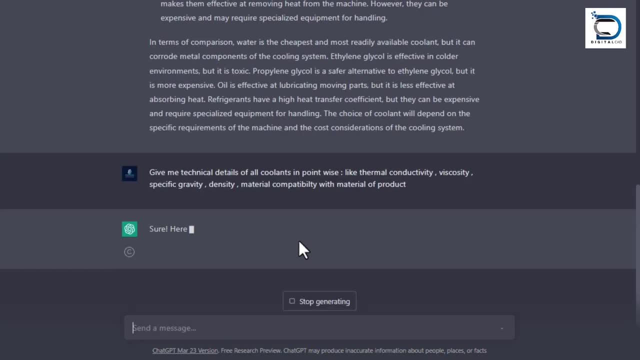 ChatGPT can provide data on specific heat thermal conductivity and viscosity of each coolant, as well as their boiling and freezing point. ChatGPT can also provide the insight into advantage and disadvantage of each coolant, such as cost availability and environmental impact. 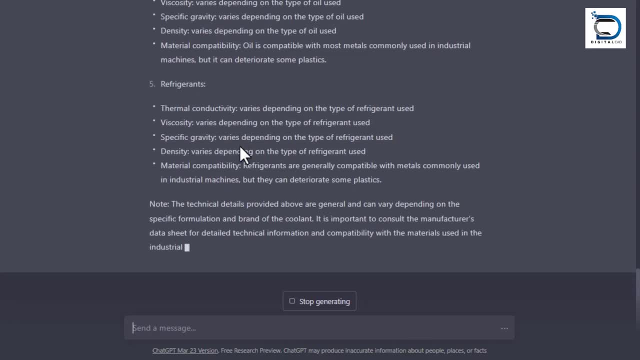 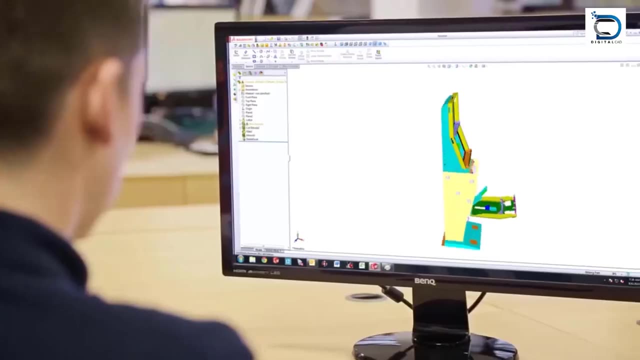 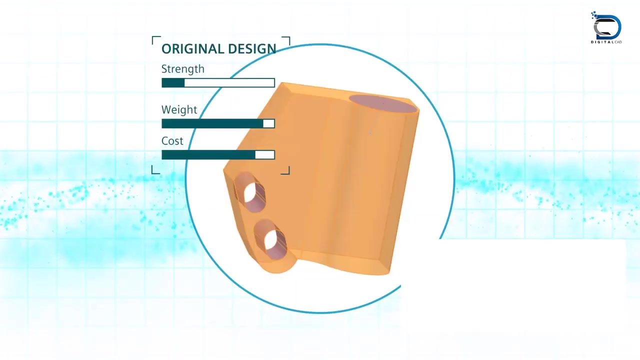 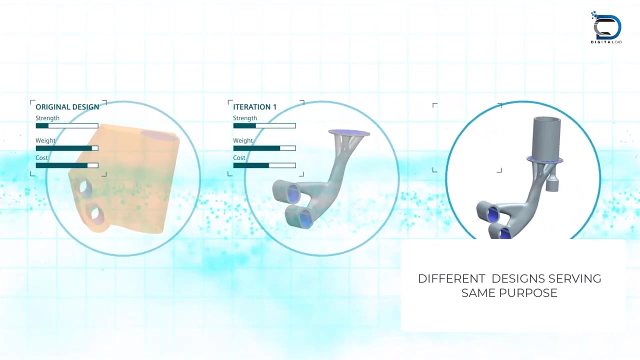 With this information, engineer can make an informed decision about the best coolant to use for system ensuring optimal heat transfer efficiency. Next up is Design. ChatGPT can help mechanical engineers generate ideas and explore various design options. For example, a mechanical engineer working on a new product can make ChatGPT to provide insight and suggestion for optimizing the design and improve performance. 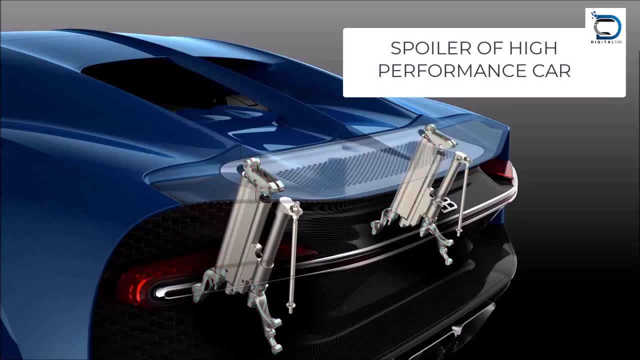 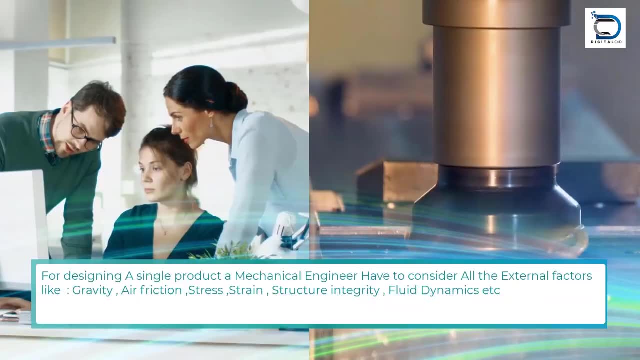 Example: Assume that Mechanical Engineer working on a new product can ask ChatGPT to provide insight and optimising the design to improve performance, reduce cost and specific application. For instance, mechanical engineer designing a high-performance racing car, The engineer needs to optimize the 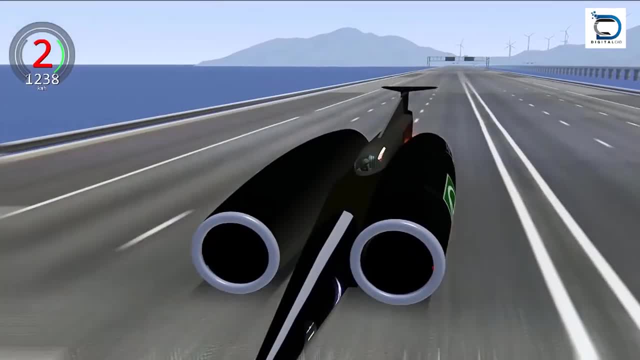 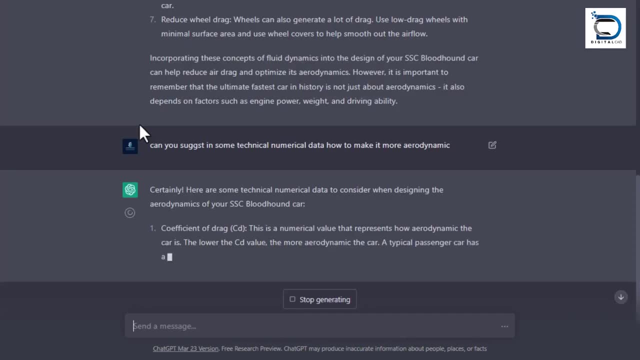 car aerodynamic to reduce drag and fuel efficiency. The engineer can ask Chad GPT to provide insights and suggestions for improving the car design. Chad GPT can provide the data on air flow characteristic of different body shape and configuration, as well as insight into effect. 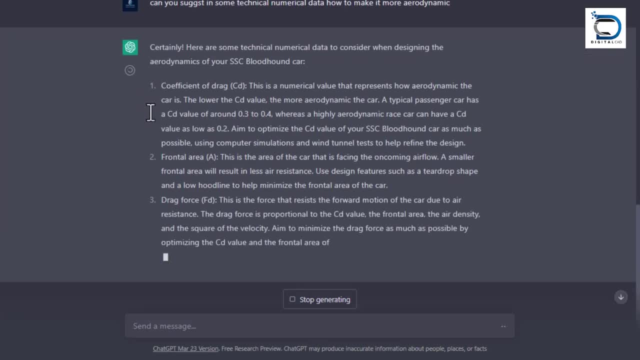 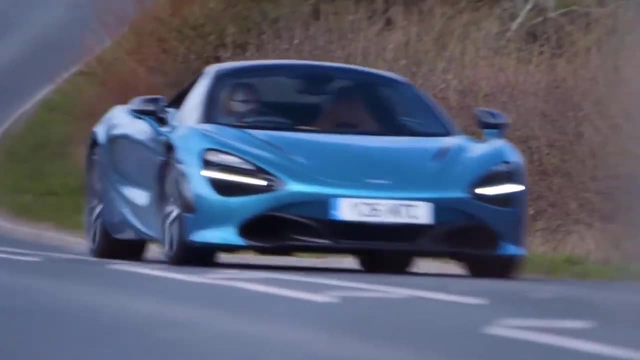 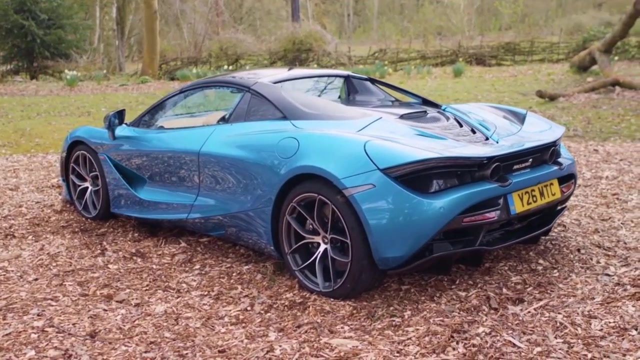 of various design elements, such as spoilers, diffuser air intakes. With this information, the engineer can explore various design options and make informed decision about the best approach to optimize the car's performance, ensuring competitive advantage on the racetrack. With Chad GPT help, the engineer can create a prototype that meets all the design criteria. 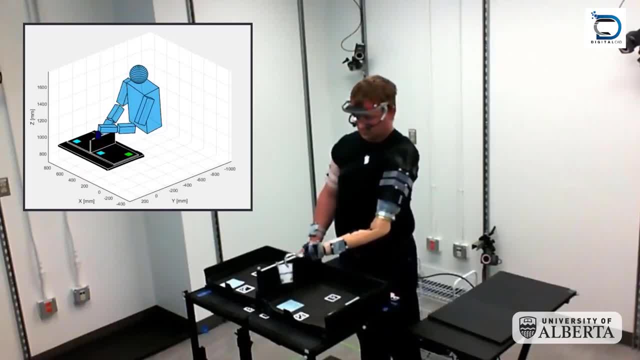 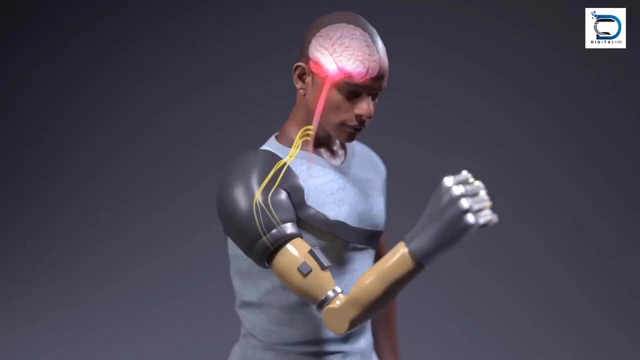 For example, let's consider a mechanical engineer designing a new prosthetic hand. The engineer needs to create a prototype that can mimic the complex movement and dexterity of a natural hand, while being lightweight, comfortable and easy to use. The engineer can also create a prototype that can mimic 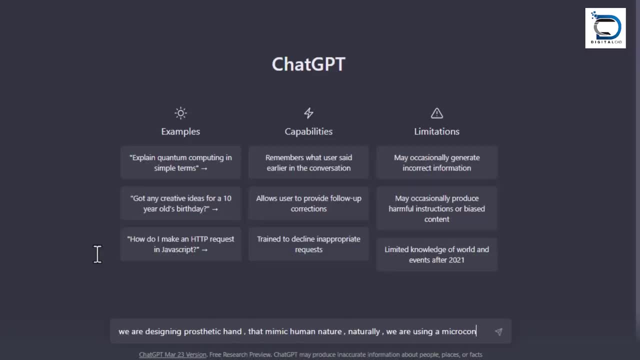 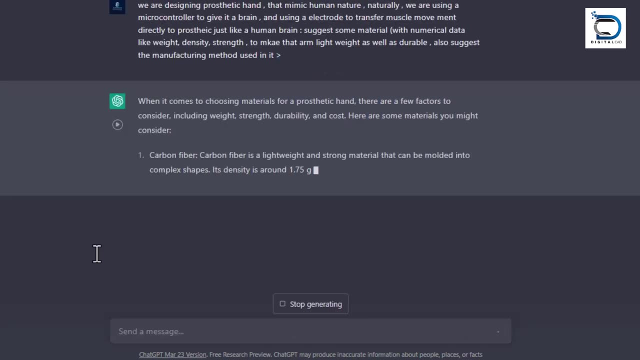 the complex movement and dexterity of a natural hand, while being lightweight, comfortable, comfortable and easy to use. The engineer can ask Chad GPT for suggestions and insight on the best material, manufacturing techniques and decision features to use in creating the prototype. Chad GPT can provide the data on mechanical properties of different materials. 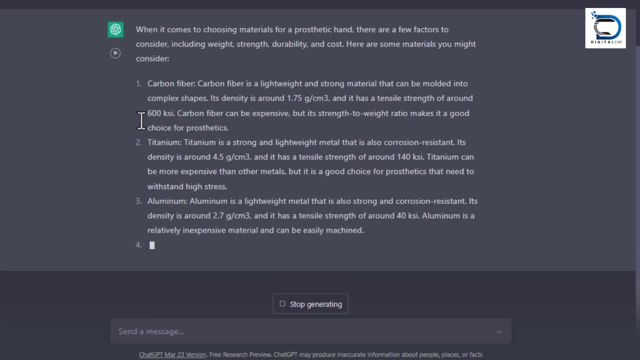 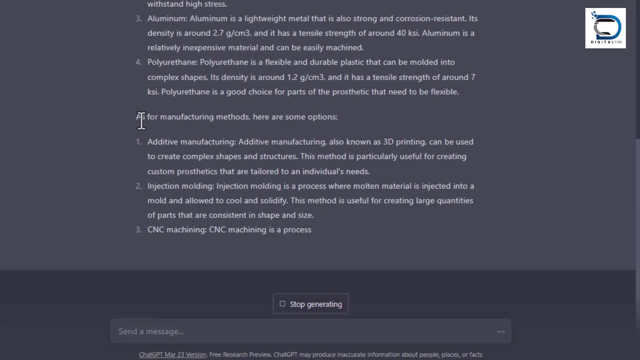 such as strength, flexibility and toughness, as well as the insight into the latest advancement in manufacturing technology, such as 3D printing or CNC machining or injection molding. Based on this information, the engineer can create a 3D model of prosthetic hand using the CAD software. 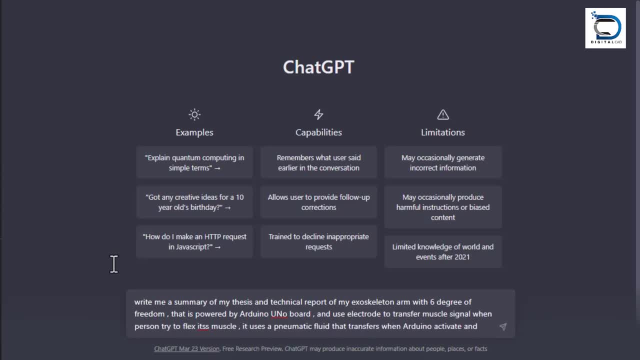 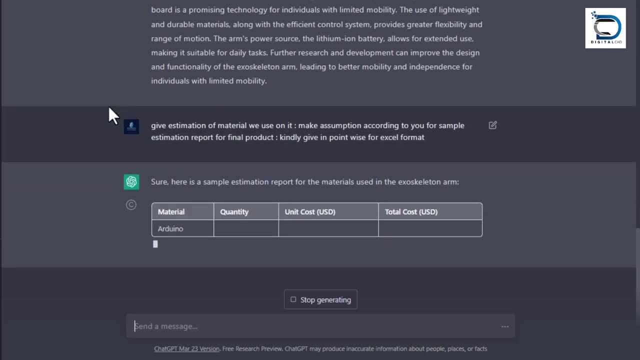 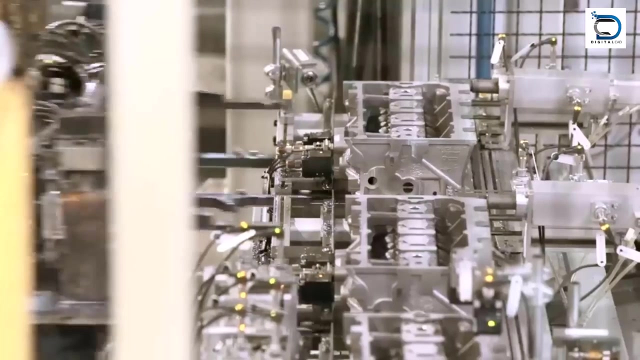 and perform simulation. Chad GPT can also assist mechanical engineers with writing technical reports, design specifications and other documents. Mechanical engineers can provide the necessary input and Chad GPT can help with organizing and structuring the information. Since we are in the age of Industry 4.0, in this age it is needed to provide every machinery. 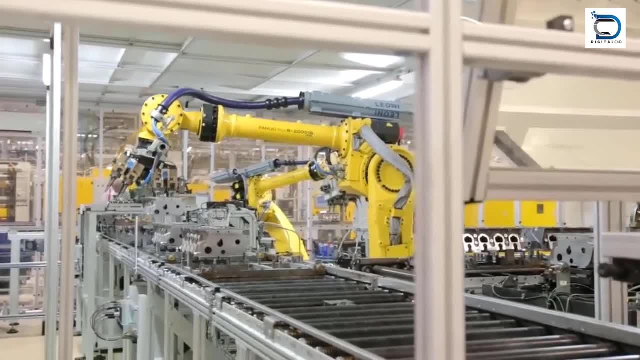 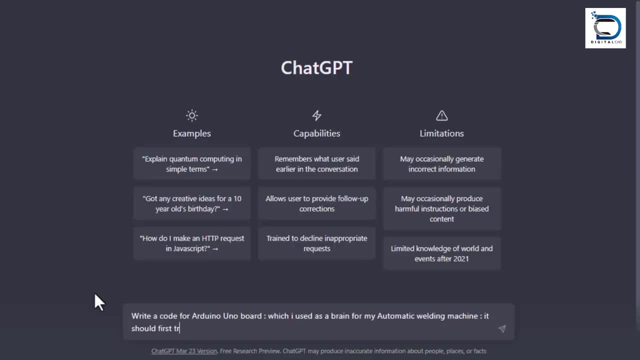 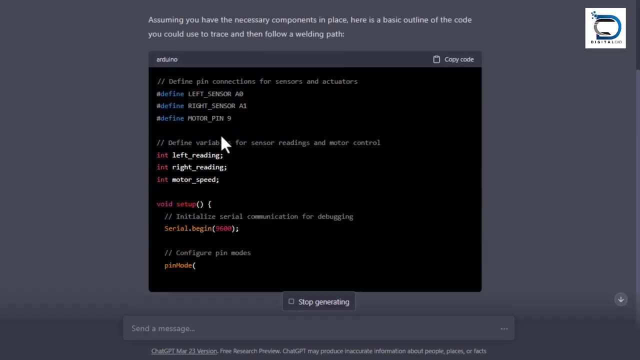 with the automation technique. For providing the automation technique we need different technologies, such as microcontroller, to grip the bayne to our machines. but in microcontroller we need a special programming and that programming- we can also do that with the help of Chad GPT. mechanical engineers can ask Chad GPT to write a code for. 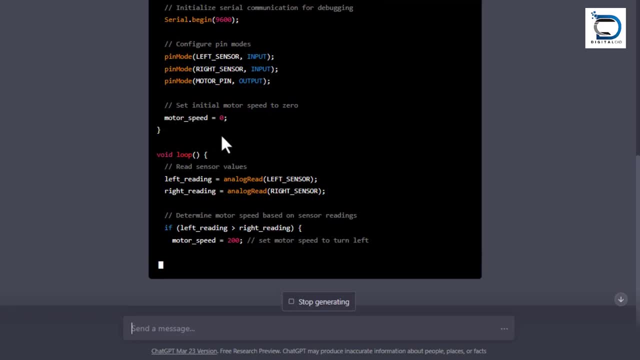 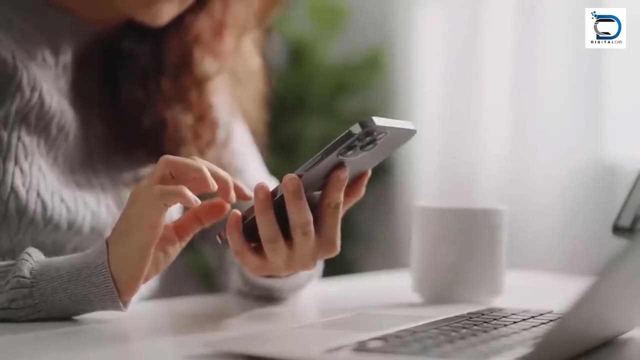 different tasks, such as automatic welding. it will write the code in just a few seconds. We just copy the code, upload into microcontroller and then our task is complete. In conclusion, Chad GPT can be a valuable resource for mechanical engineers. it can help with research.